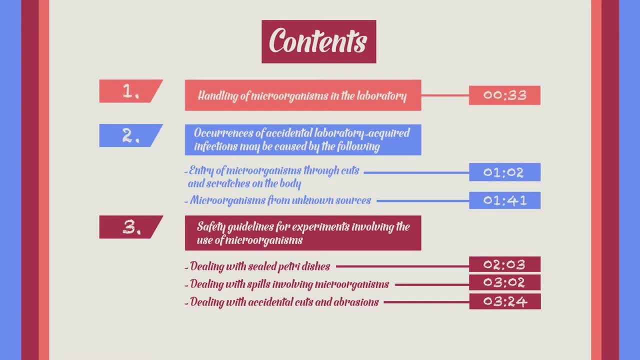 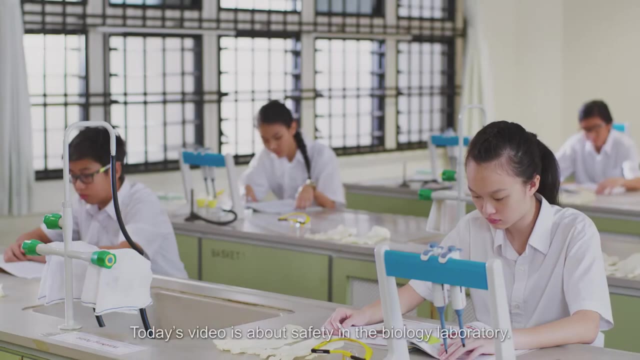 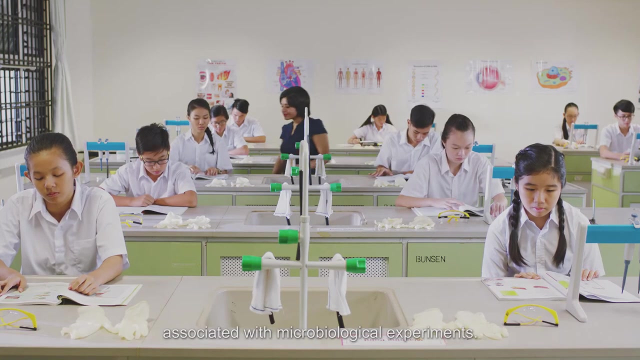 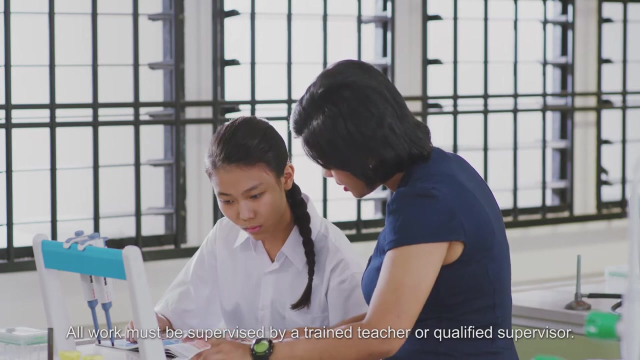 Today's video is about safety in the biology laboratory. Teachers and students must be aware of the importance of safety precautions associated with microbiological experiments. All work must be supervised by a trained teacher or qualified supervisor. Microorganisms are a potential hazard to persons performing microbiological experiments. 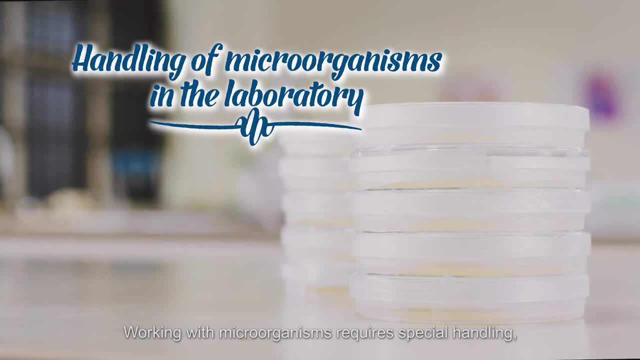 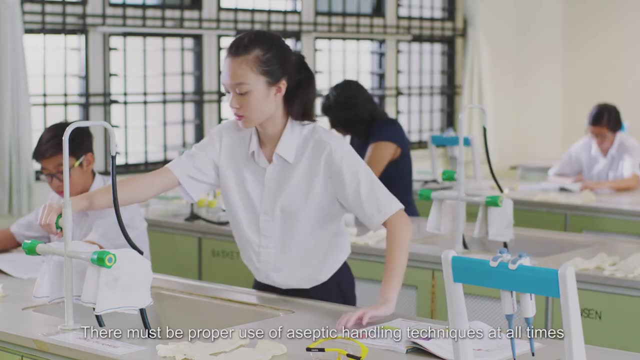 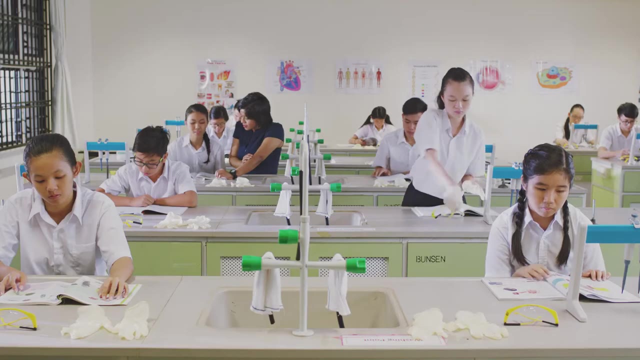 Working with microorganisms requires special handling, storage and disposal techniques. There must be proper use of aseptic handling techniques at all times, such as wearing of gloves and proper washing of hands. Here are some scenarios where accidental laboratory-acquired infections may occur. 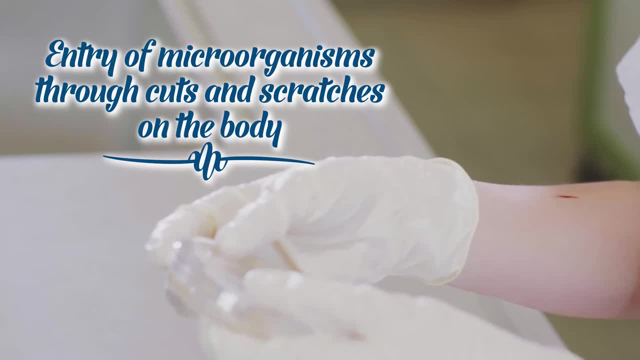 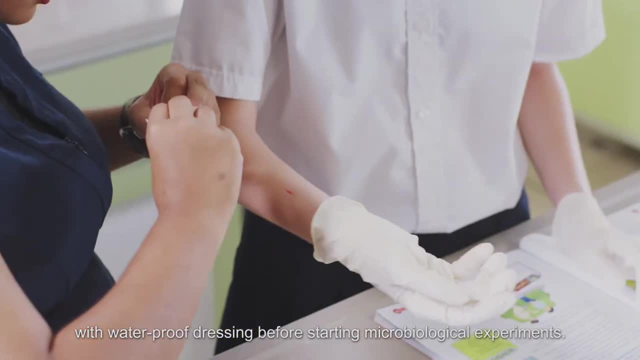 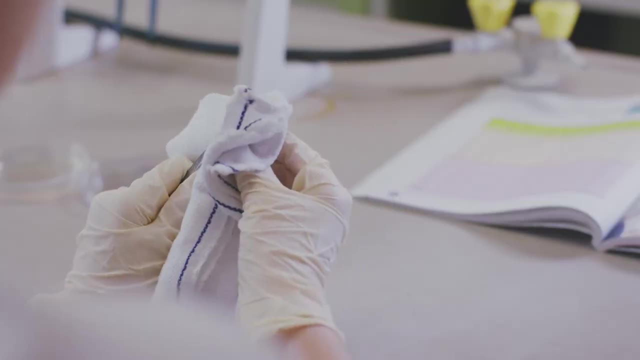 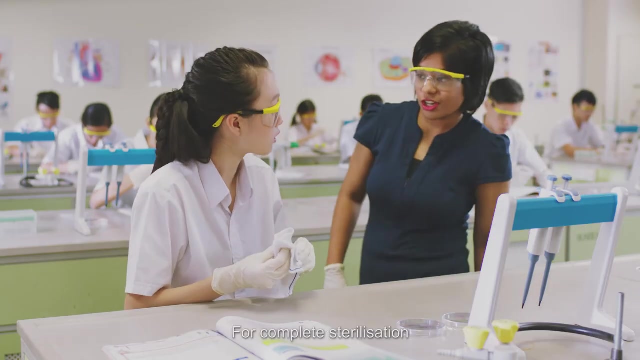 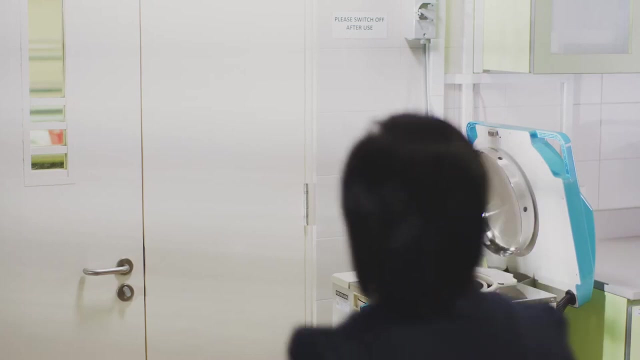 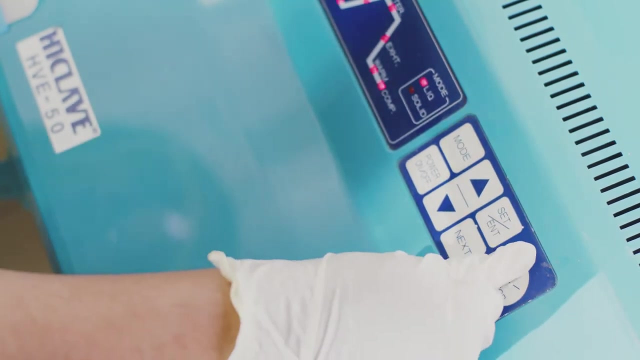 All cuts on the body surface should be covered with waterproof dressing before starting microbiological experiments. Liquid disinfectants and germicidal agents generally have limited effectiveness For complete sterilisation. all apparatus used in microbiological experiments must be autoclaved. Only known microorganisms from recognised suppliers should be used for inoculation. 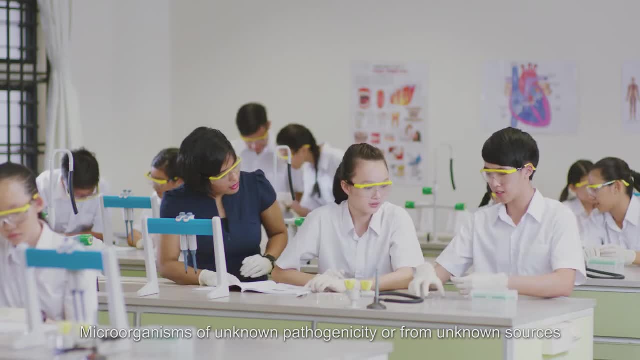 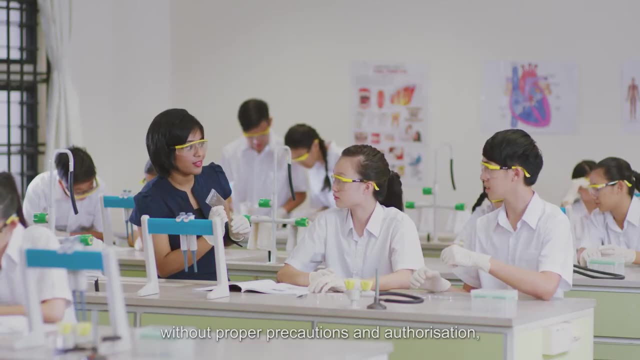 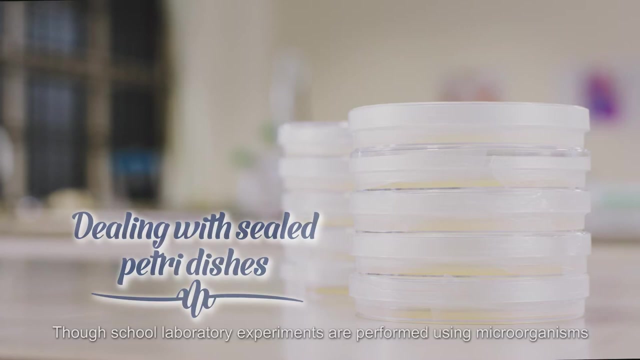 Microorganisms of unknown pathogenicity or from unknown sources should not be brought to the laboratory. They should not be brought into a school laboratory without proper precautions and authorisation, For example, attempts to isolate unknowns from soil culture, Though school laboratory experiments are performed using microorganisms that are unlikely to cause disease in humans and animals. 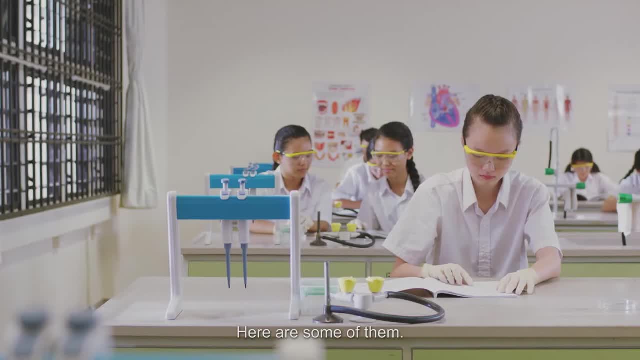 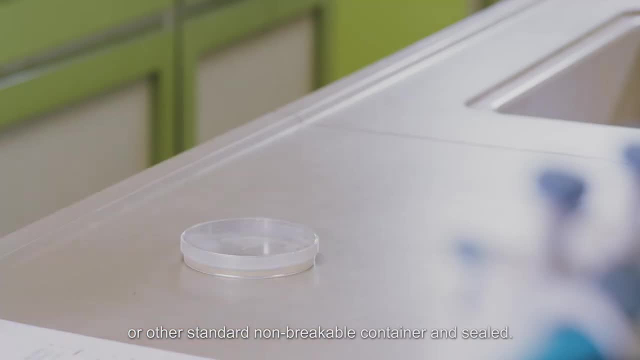 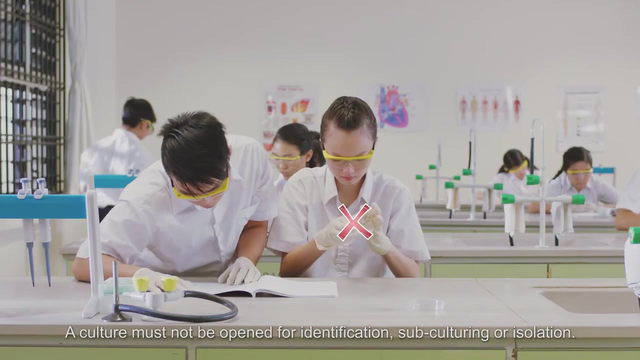 there are still safety guidelines to be followed. Here are some of them. The microorganism is cultured in a plastic petri dish or other standard non-breakable container and sealed. A culture must not be opened for identification, subculturing or isolation.